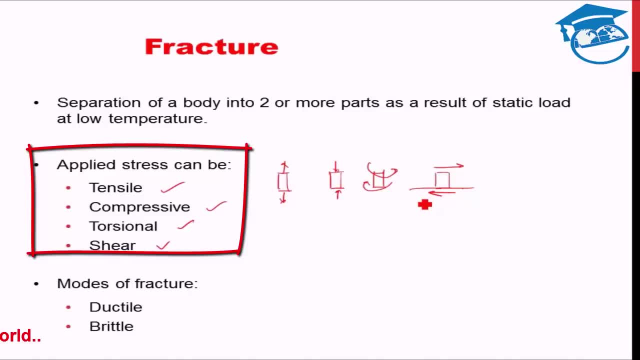 that can exist And all of them can effect fracture. All of them can lead to fracture. Now fracture modes of fracture are two. One is ductile fracture, The second is known as brittle fracture. We will see in details what each of them is, But just to give you, 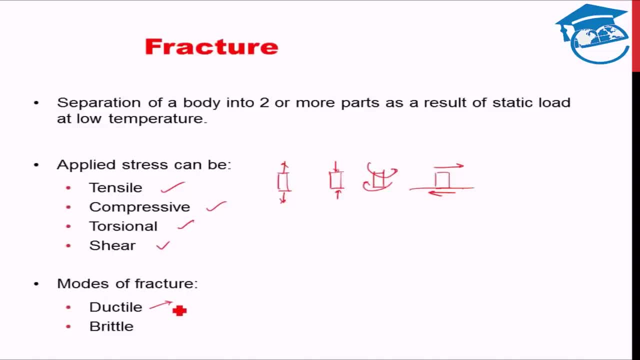 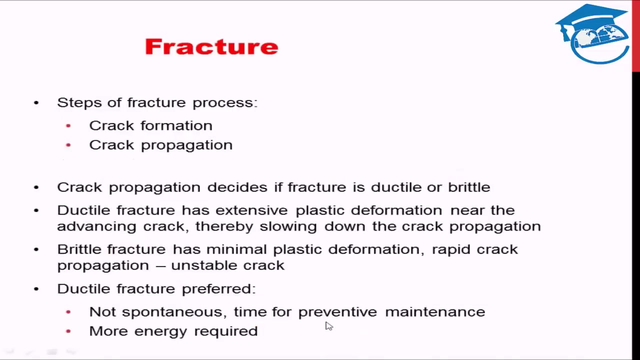 an idea. ductile fracture has plastic deformation associated with it. Brittle fracture has no. brittle fracture has no, or very less plastic deformation. Fine Now, how does a fracture take place, Similar to fatigue, where you had to have a crack, and that crack basically propagates, resulting in fatigue failure. fracture also needs to. 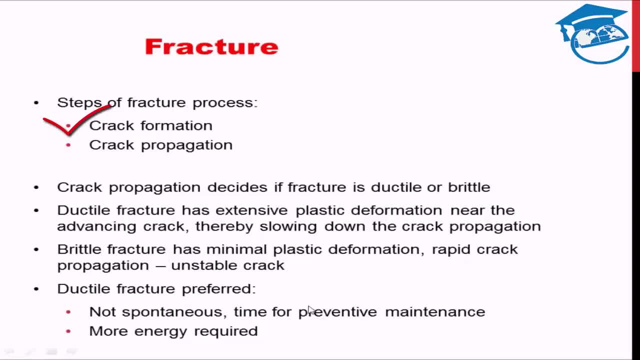 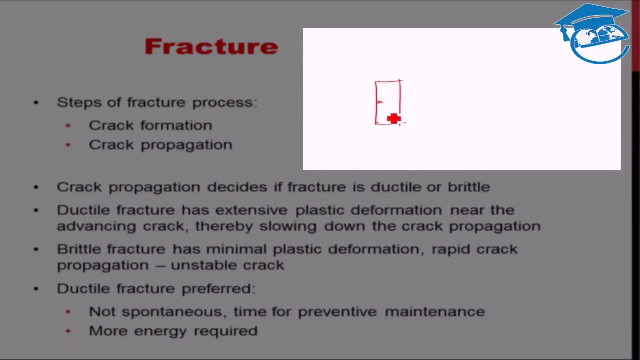 have a crack initiation or crack formation and crack propagation. So crack initiates that propagates, leading to failure. Crack propagation- the method by which crack propagates, basically decides if a fracture is ductile or brittle. Right Suppose we have a body and somehow a crack is formed on the body. This crack 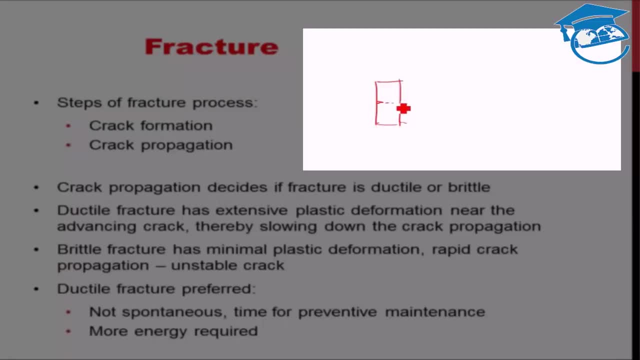 needs to travel from this end throughout the body. It should traverse throughout the body for the fracture to be effective, like the material to collapse into two pieces, Isn't it? Now, how does this crack propagate through the body? That will define whether the fracture type mode is ductile or the fracture mode. 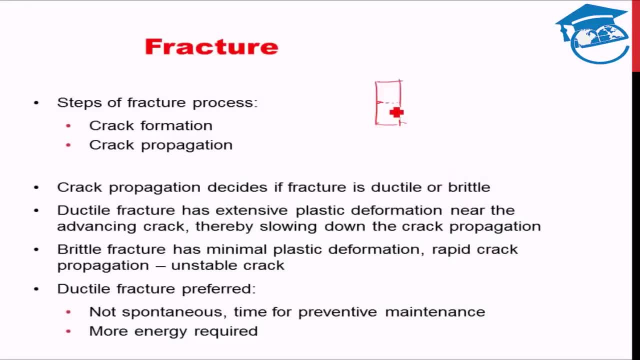 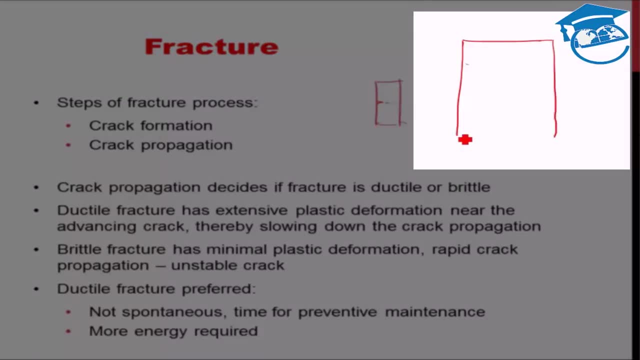 is brittle fracture. What will happen in ductile fracture is that ductile fracture has extensive plastic deformation. Ok, So let's draw a bigger diagram. So if we have a fracture notch like this During propagation of crack, what will happen? The front of crack, the area just before the crack, just in front of the crack, will have extensive plastic deformation. 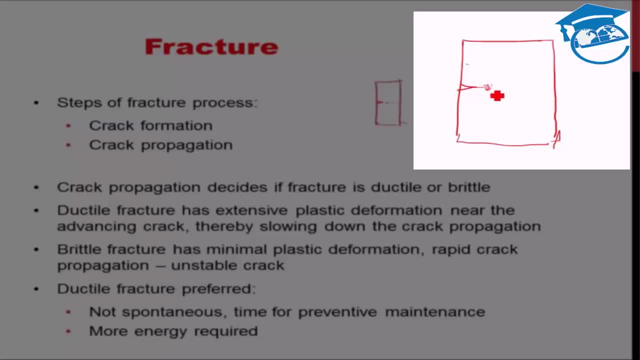 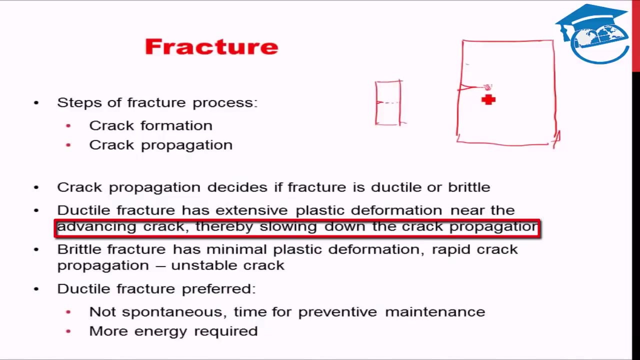 Okay, so that will take up a lot of energy for the material just in front of the crack to plastically deform. There will be strain over there right And the advancing crack as a result will be slowed down due to extensive plastic deformation. 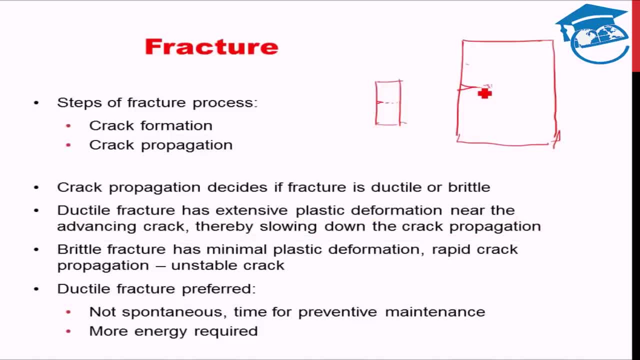 Because obviously a lot of energy is going into the plastic deformation of the front region, So crack cannot just pass through that region. It requires time for the energy to plastically deform the region Okay, And also the amount of energy is going to the front of the crack. 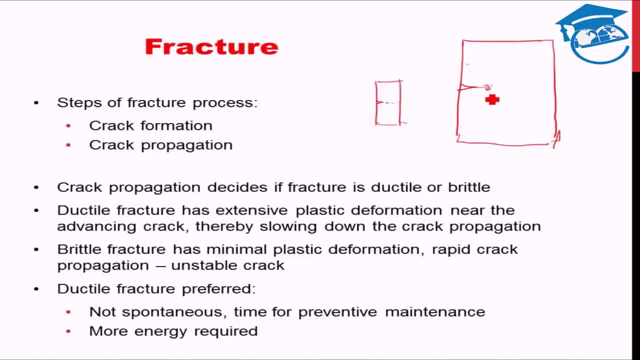 Okay, And also the amount of energy is going to the front of the crack. So the amount of energy required for a ductile fracture will be more right, Because a lot of plastic deformation needs to take place for the crack to keep on propagating. 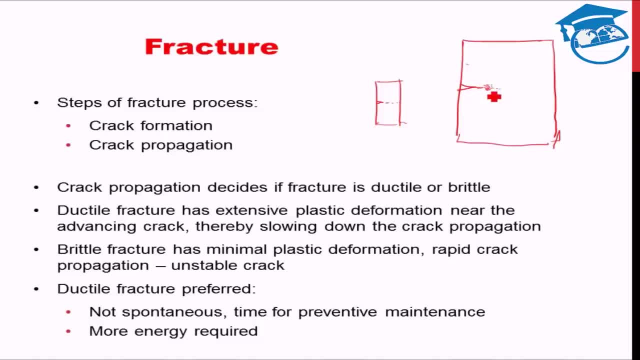 Therefore, ductile fracture is able to absorb a lot more energy than a brittle fracture, Because brittle fracture has no or minimum plastic deformation. When there is no plastic deformation, only elastic deformation is required. When there is no plastic deformation, only elastic deformation is required. 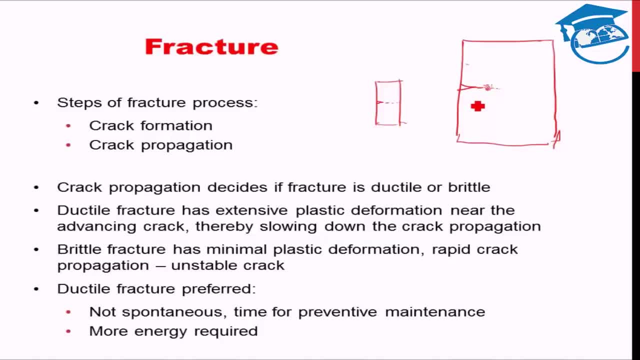 Then amount of energy absorbed will be much less. Thereby the crack propagation will be much more rapid. Okay, And this rapid crack propagation, in the case of brittle fracture, is known as unstable crack propagation, Because there is nothing to stop the crack, right? 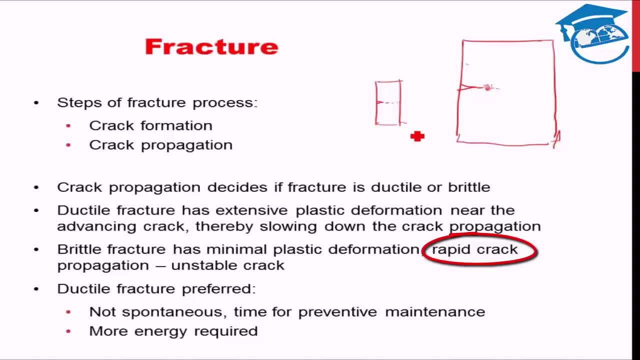 There is no restoring force to slow down the crack propagating. It will just initiate and within almost no time the crack propagates through the material, causing fracture, Almost instantaneous fracture in the case of brittle material Right. So that is the basic difference between ductile fracture and brittle fracture. 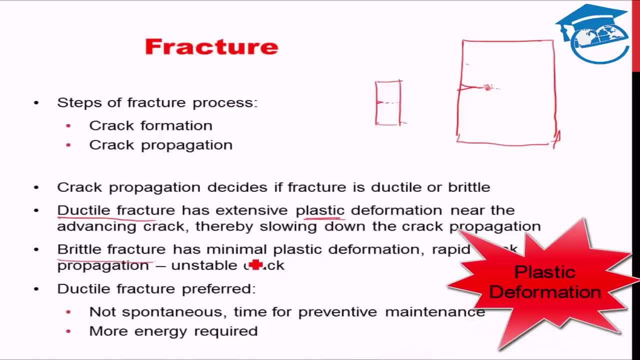 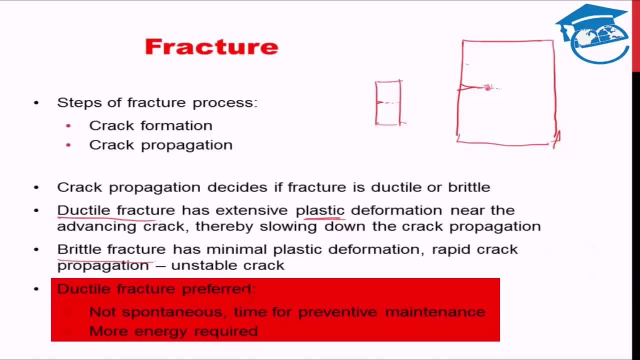 Plastic deformation. That is the key word. Now, why is the ductile fracture preferred? Ductile fracture is the kind of fracture which engineers prefer for a material to have. Why is it so? Because it is not spontaneous, It is non-spontaneous. 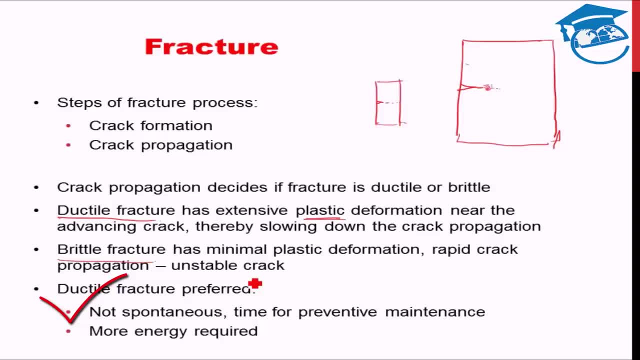 Thereby there is more time for preventive maintenance. There is scope to identify that the material is going to fracture beforehand, Because the fracture is going to take a lot of time to actually happen, Whereas in brittle fracture, the fracture being spontaneous and immediate, it can be catastrophic. 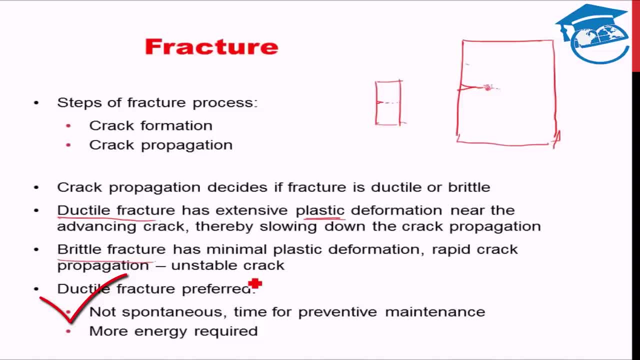 Therefore ductile is thought or kind of preferred fracture. It is the evil, but it is the preferred evil. Secondly, ductile fracture, as I said, requires much more energy than brittle fracture, So it can last lot longer, Much harsher. 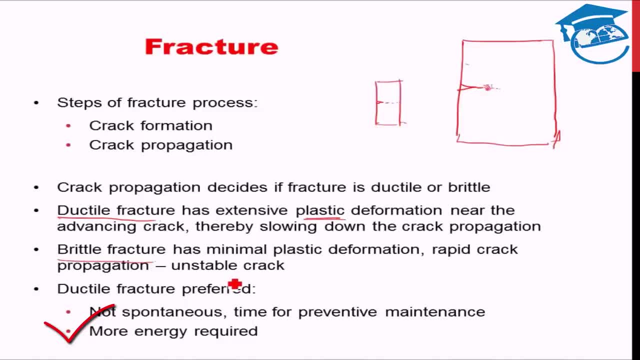 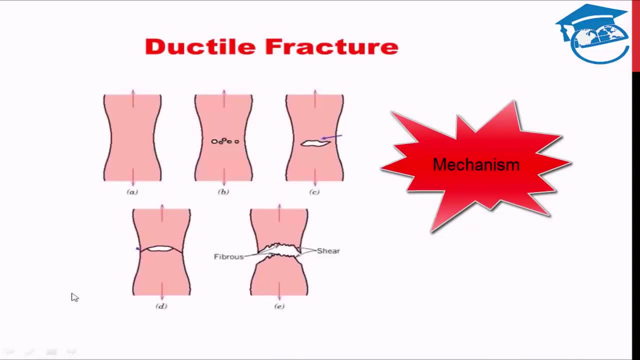 Much harsher conditions than brittle material is undergoing brittle fracture. That's why ductile fracture is the preferred mode of fracture for engineers. Now let us see the mechanism of ductile fracture. Exactly, how is the ductile fracture happening? What is happening is that you apply the load. 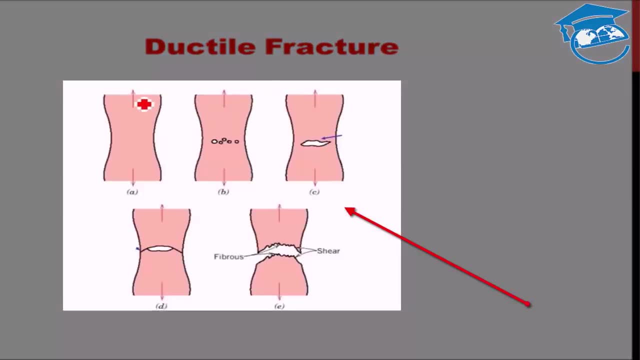 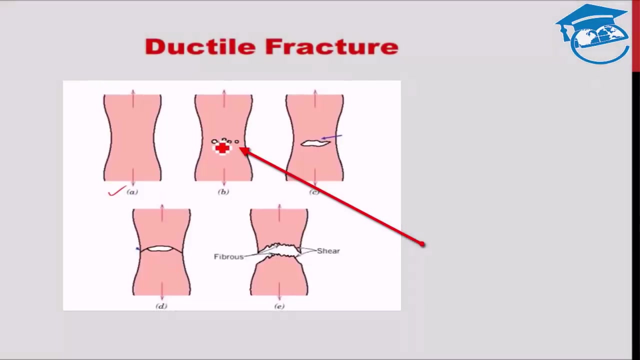 Initially, the initial loading Loading will go into creating neck. The neck formation will take place As shown in stage 1.. And beyond that, what will happen? We will start getting small micro-voids, at the central region may be, or at the edges also. 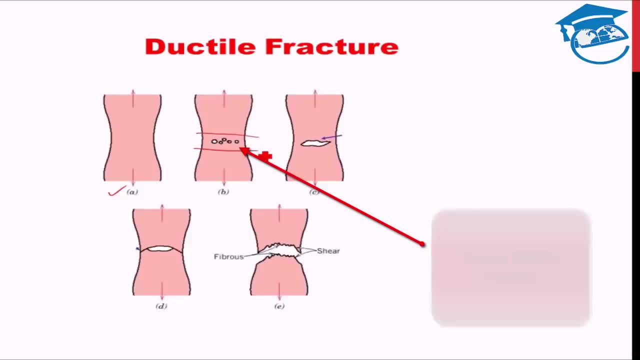 Mostly at the central region, In the region where the neck has formed. These will be micro-voids which can be observed under a microscope. Third stage Is coalescence of those micro-voids. The micro-voids comes together and becomes sufficiently large. 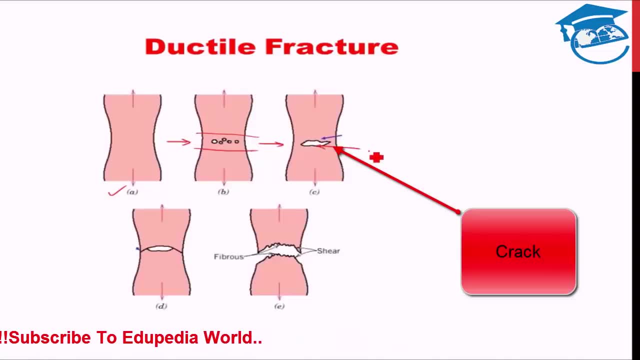 And then it becomes a proper crack Right And once it reaches a certain length, A sufficient length, Then basically shearing will happen. after that Shear forces will take over, And Then something like this, And shear forces are maximum at 45 degree: 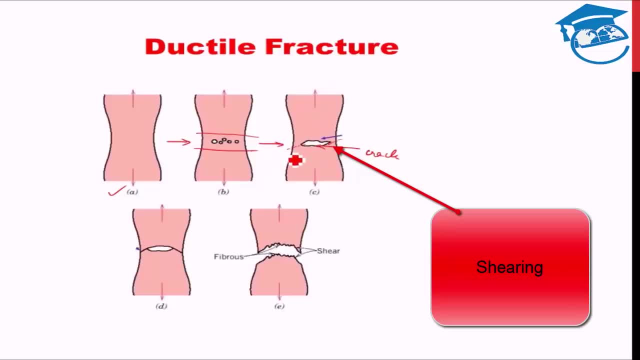 This is tensile force. Shear forces are maximum at 45 degree to tensile forces. Therefore, the last stage of crack propagation, The last steps, will see a 45 degree angle And this will be the fibrous region. The central region will be fibrous crack scenario. 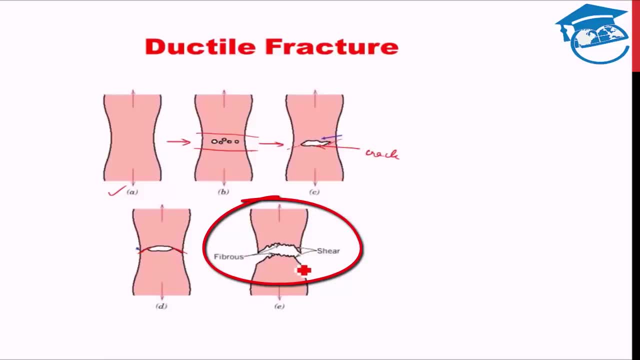 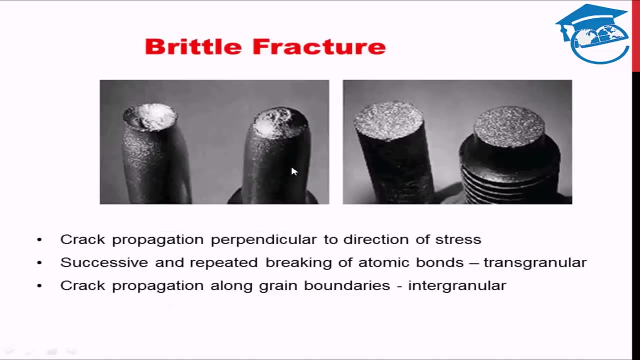 And over here will be the shear crack scenario. So this is the overall ductile fracture mechanism. In the brittle fracture mechanism, Next page, I will show you two figures, One for ductile and one for brittle. Let's see: Okay, So this is a ductile fracture. 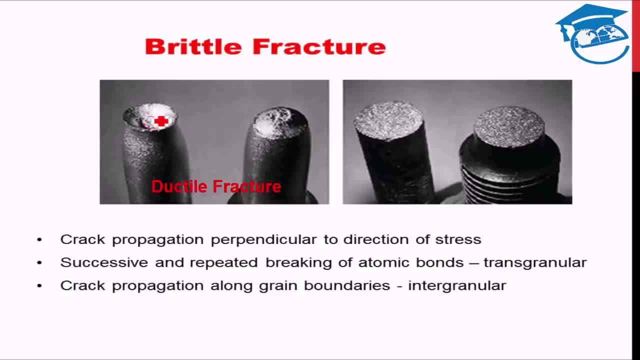 You can see that this region is the fibrous region And this region is the shear region. It's almost at 45 degree. This is the other end. So this is 45 degree Here, 45 degree, And this is the fibrous region. 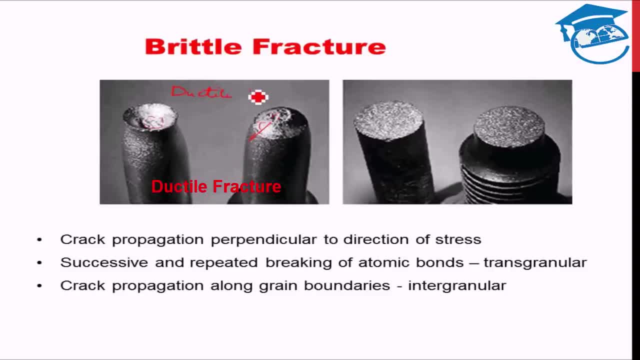 This is my ductile fracture, Whereas in brittle fracture what you will see is Brittle fracture. What you will observe is that the surface, The crack surface, The surface has cracked Almost perpendicular to the loading. So if the loading was like this: 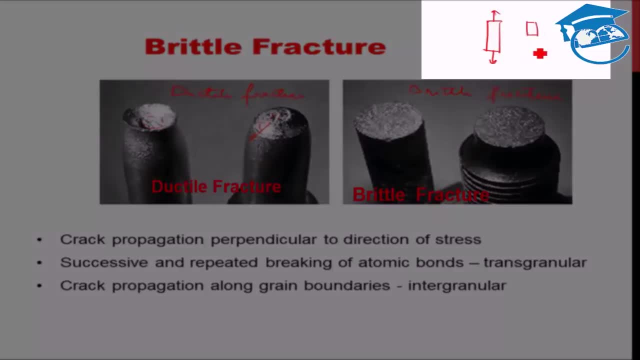 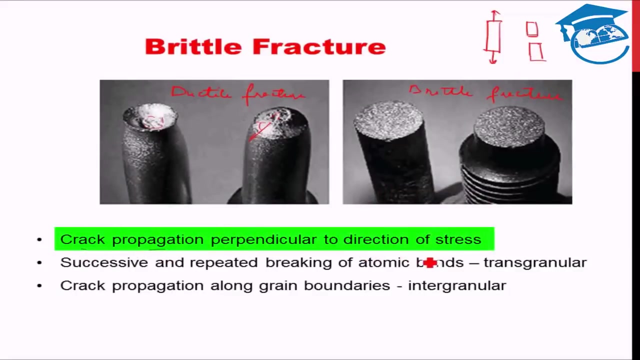 The resultant Material which we obtain after cracking will be like this: It's almost perpendicular to the load Right. The crack propagation is perpendicular to the direction of the stress. Also, in brittle fracture what happens Is actually there is successive breaking of bonds. 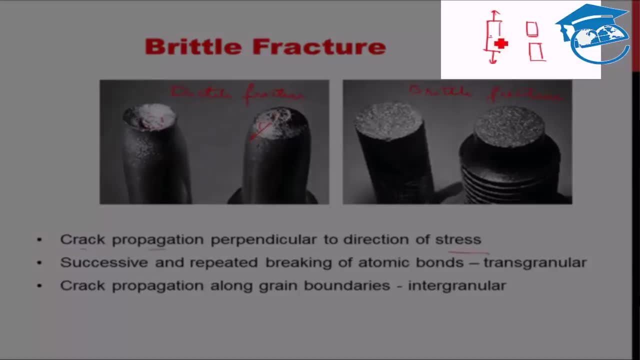 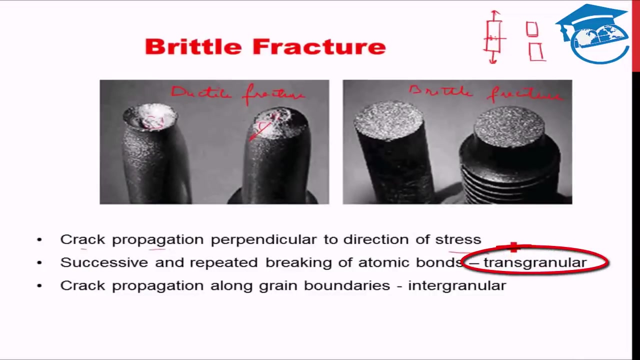 So basically, Bonds will start to break, rupture And those rupturing bonds keep on breaking, breaking, breaking And the whole fracture occurs, And this is kind of transgranular Through grains. Okay, Alternatively, what can happen is that crack propagation can also. 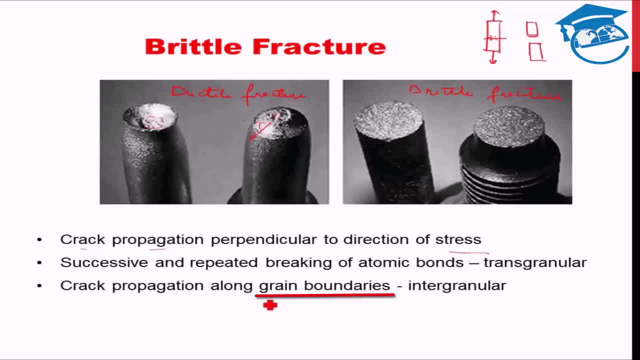 Occur along the grain boundaries. In that case the crack will not propagate Through the grains, Rather it will propagate along the grain boundaries And then That type of brittle fracture will be known as intergranular fracture. Transgranular is through the grains. 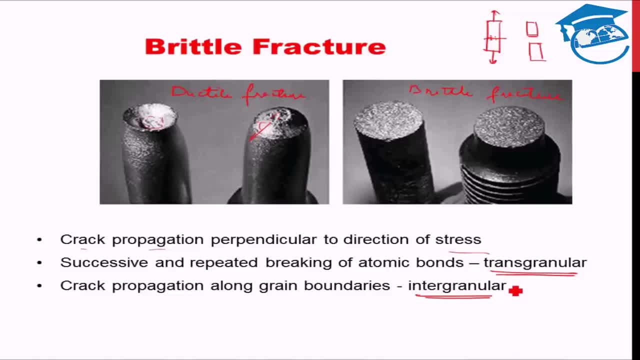 Intergranular is Between the grains Or along the grain boundaries. Okay, So We have seen the two modes of fracture, That is, Ductile fracture And the brittle fracture. Here A lot of plastic deformation is taking place. 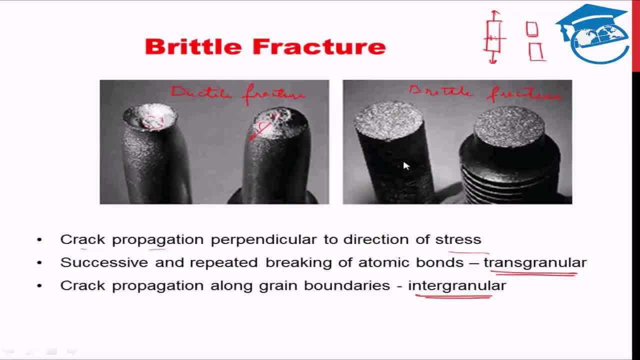 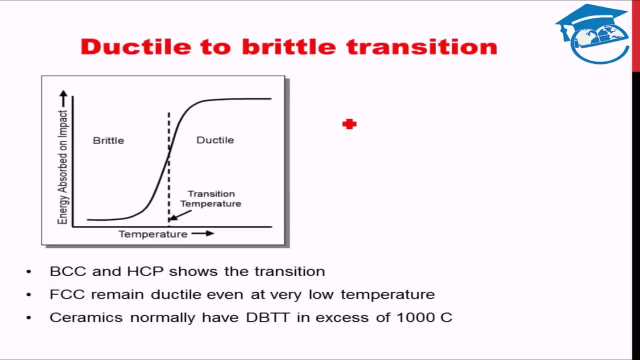 Here, plastic deformation is almost non-existent. Now, This Is something Which I have discussed. In the first, Very first lecture, When I was introduced you to the sinking of Titanic, If you remember, I told you something about ductile to brittle transition. 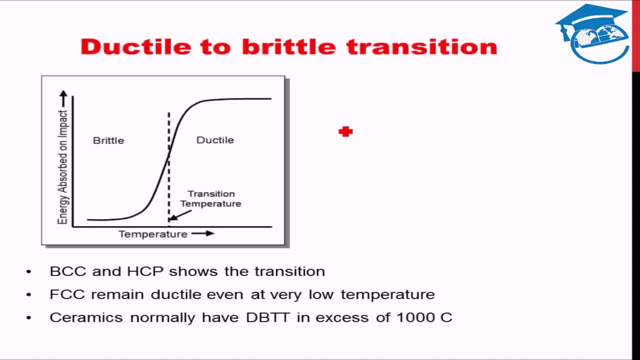 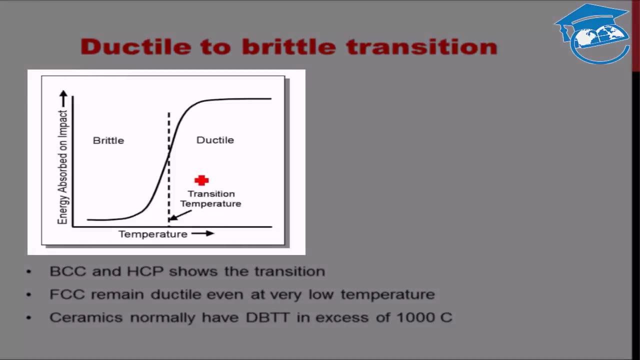 What happens is the fracture mode, Where Changes from ductile fracture mode, Which is the preferred mode, To brittle fracture mode. On lowering the temperature, There is a transition temperature Below which The Mode of fracture is brittle, Above which 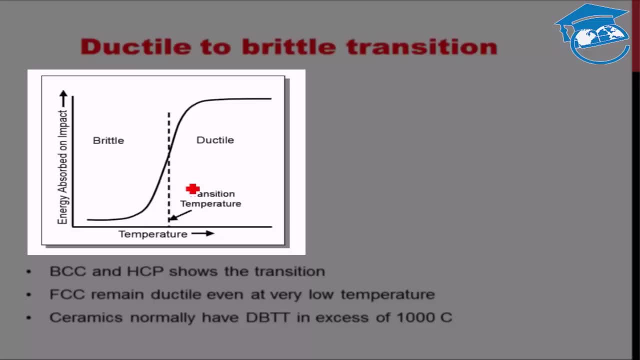 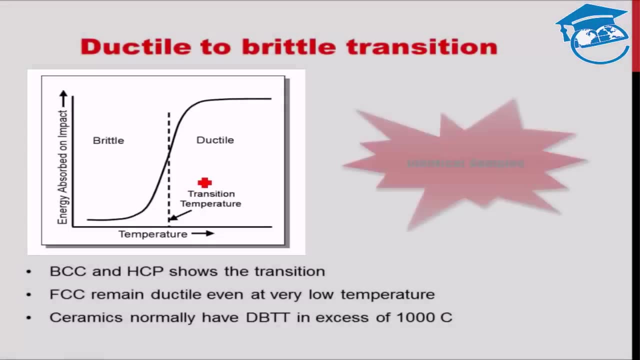 The mode of fracture is ductile. How do we find What is the temperature? What we do Is basically We create Identical samples, Many identical samples, And We Break them By impact. I have not discussed. 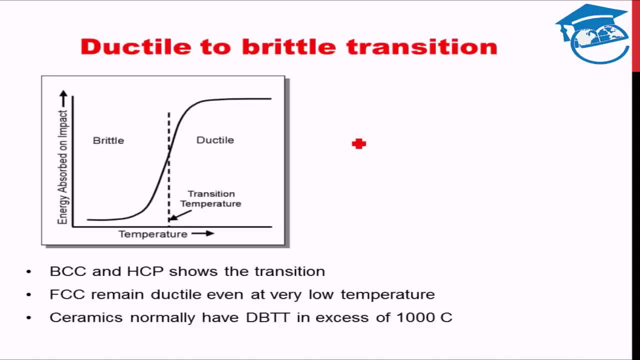 About the different impact test. But Then There is something Known as Charpy Impact test. There is Izod impact test. Those tests Can be used To Determine How much Impact Energy Is. 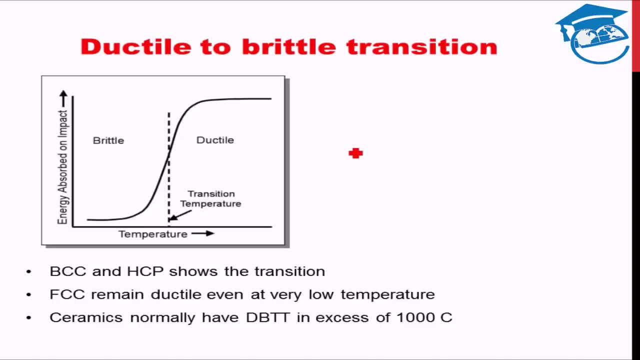 Absorbed By a material To fracture. Okay, By using those tests, What is done Is Several N number of samples- Let's say Five samples Are- Are Fractured Using the impact testing. 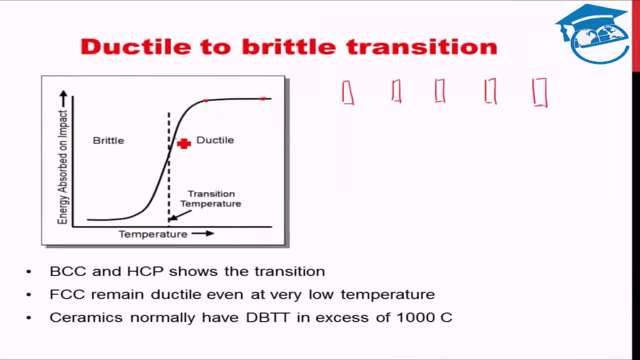 At Five Different Temperatures: One, Two, Three, Four, Five. So The Impact Testing At Five Different Temperatures, Five, And The Energy Is Noted. The 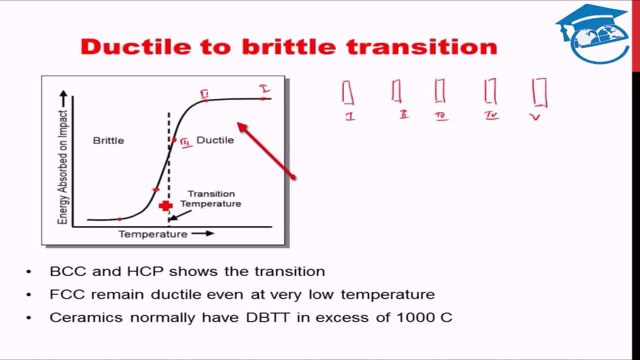 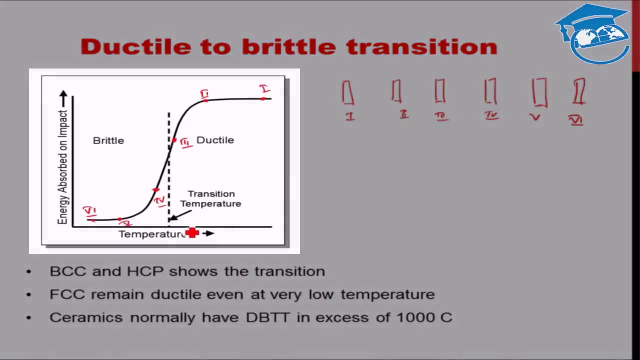 Amount Of Energy Required For Fracturing. Each Of The Sample Is Noted And It Comes Out Something Like This: Let's Say There And We'll. 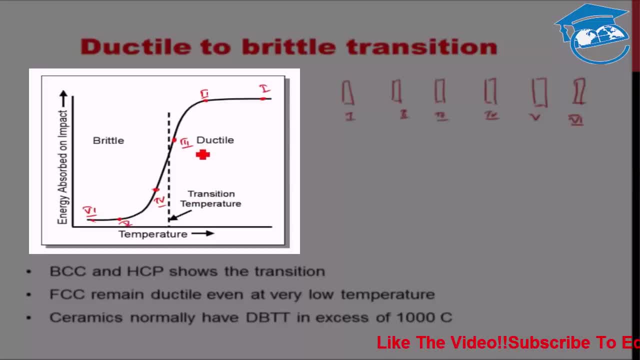 See That For Certain Materials There Will Be A Sudden Dip In The Amount Of Energy Required To Fracture It Somewhere Over Here. The 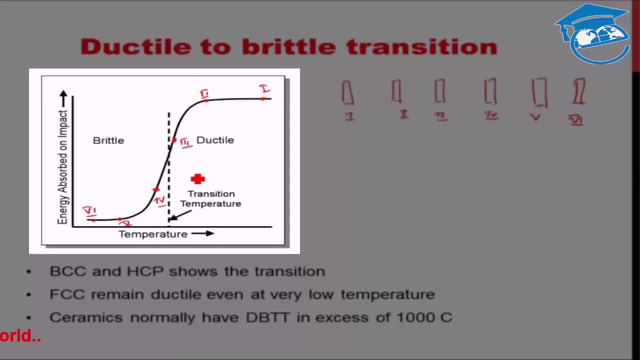 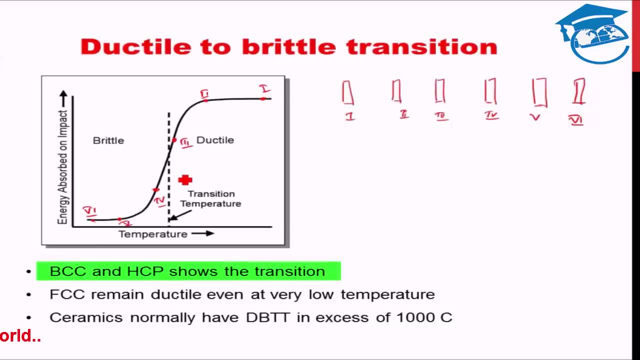 Amount Of Energy. But All Materials Will Not Have A Ductile To Brittle Transition Temperature. BCC And HCP Materials Shows Ductile To. 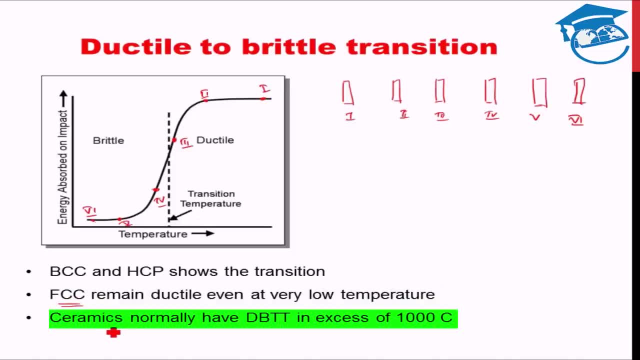 Brittle Transition Temperature. FCC Materials Normally Remain Ductile Even At Even More Than That Is Why Ceramics Normally Have Brittle Failure Right. That's. 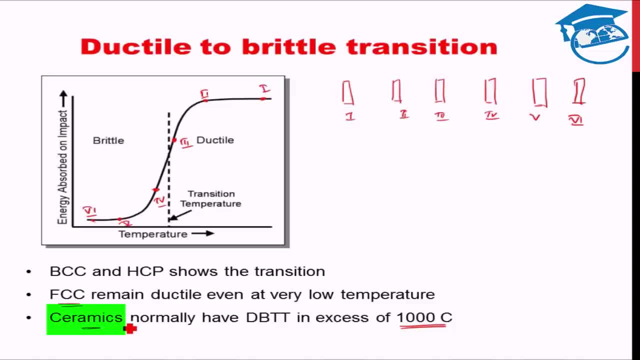 Why Ceramic Bowl? If It Falls, It Just Breaks, And The Break Surface, If You Observe, Is Component. The Steel Was Of BCC Type. 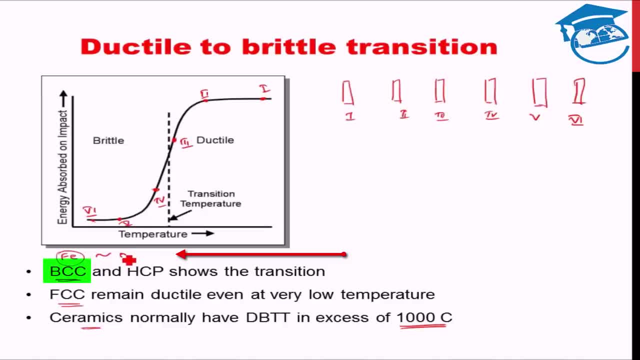 So The Ductile To Brittle Transition Temperature For That Steel, Due To The Presence Of Sulphur, Was Nearly Zero Degree Celsius, And Okay. 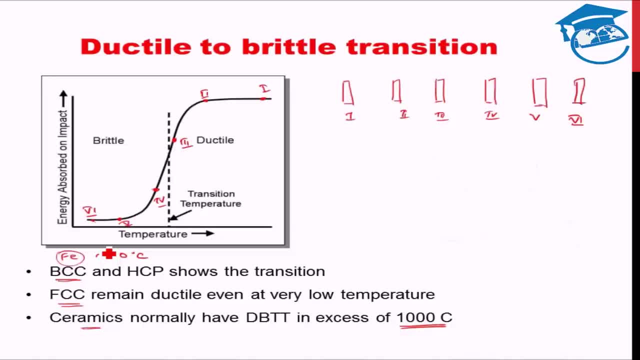 So This Gives You Interesting Idea That There Can Be Transition Between Ductile And Brittle Failure Mechanism For Fracturing. So The Idea Is: